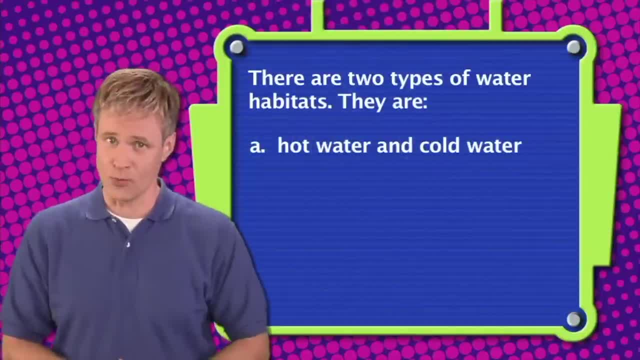 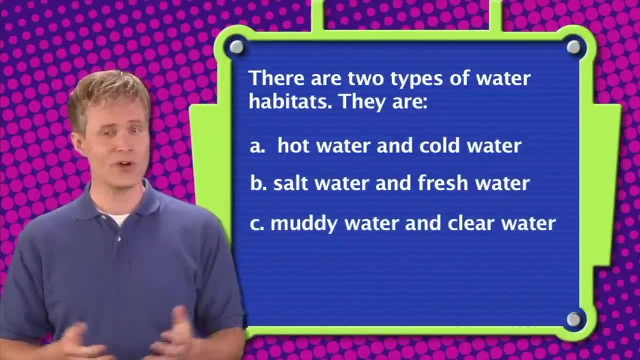 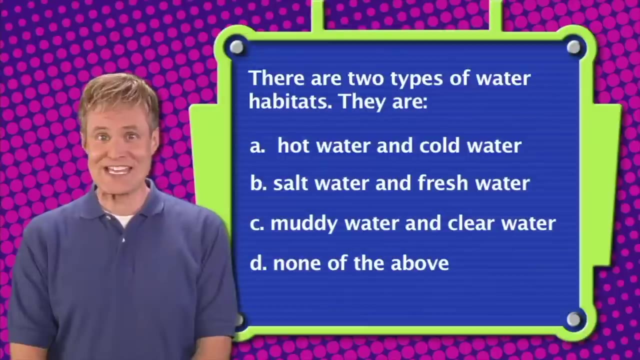 They are: A- Hot water and cold water, B- Salt water and fresh water, C- Muddy water and clear water Or. D- None of the above. The correct answer is B- Salt water and fresh water. Here's the next question. 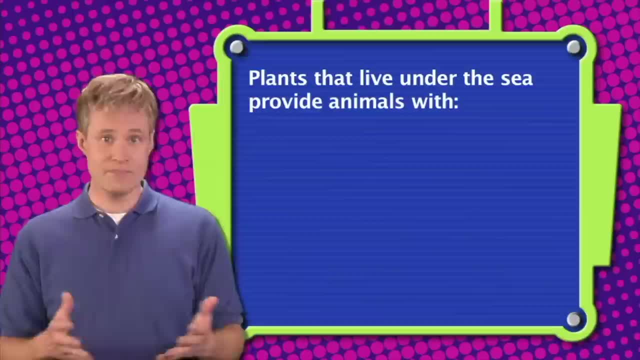 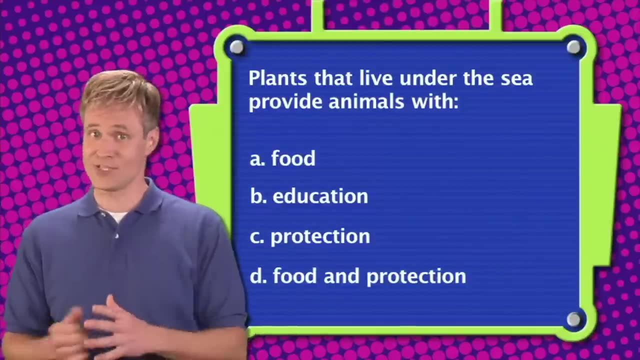 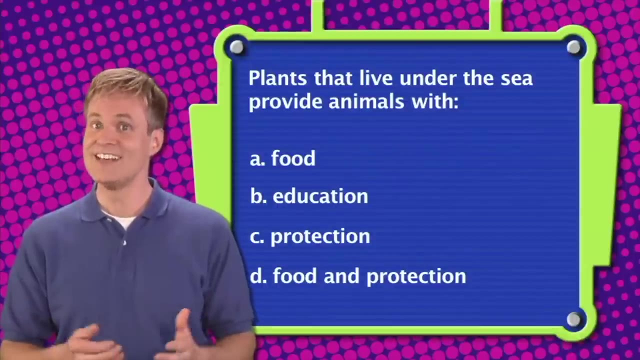 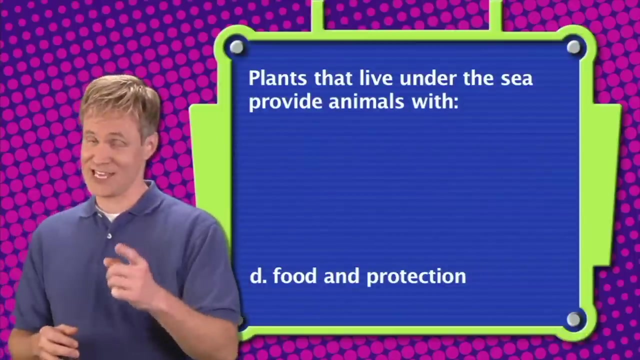 Plants that live under the sea provide animals with A- Food, B- Education, C- Protection, D- Food and protection. The correct answer is D. Plants that live under the sea provide animals with food and protection. Thank you for playing. Know Your Water Habitat. 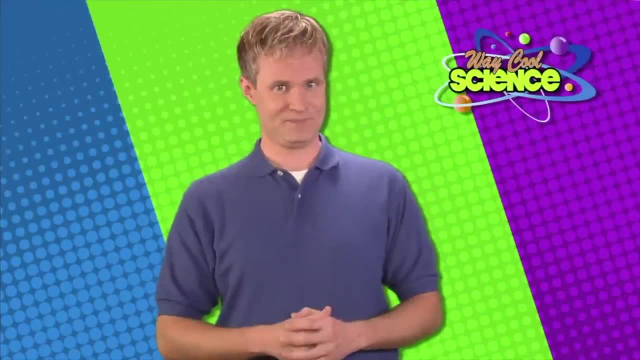 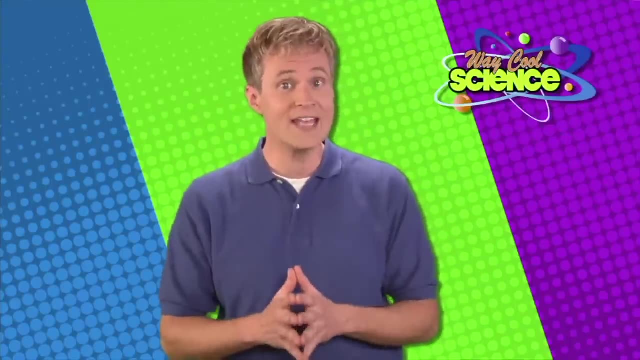 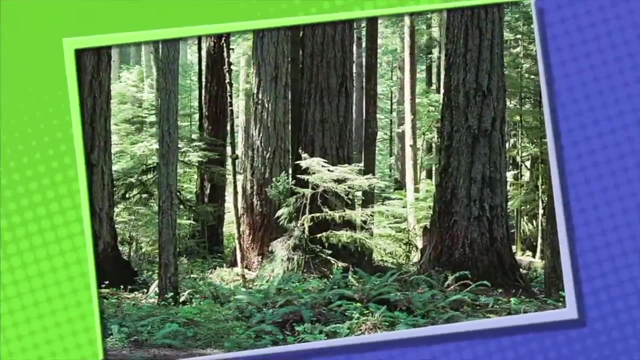 The next habitat we're going to explore is the forest. There are three different kinds of forest habitats, and each forest habitat is home to many different types of plants and animals, like lions, tigers and bears. Oh my, The first type of forest habitat is called coniferous forest. 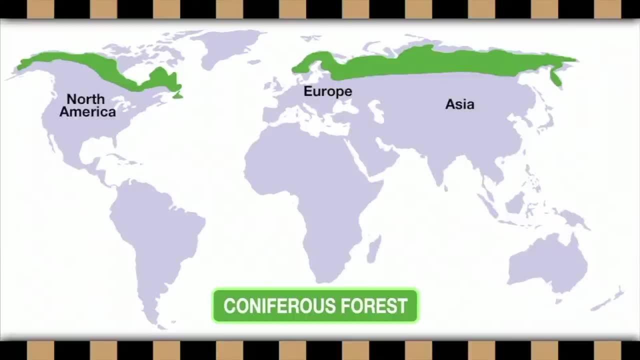 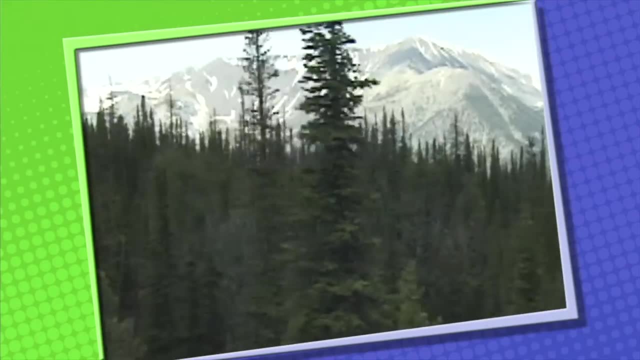 Coniferous forests are found in the northern regions of the world, on the North American continent, parts of Northern Europe and Northern Asia. Trees found in the coniferous forests, like firs and spruce, have dark green, needle-shaped leaves that stay green all year. 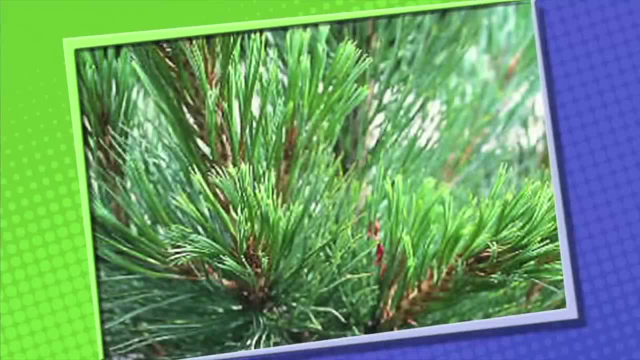 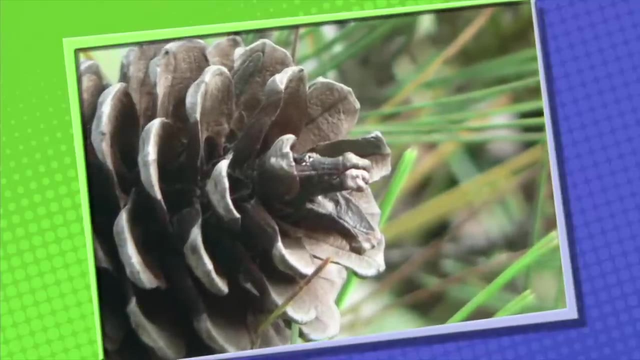 The dark green color of spruce and fir needles helps the foliage absorb the maximum heat from the sun and begin photosynthesis as early as possible. The word coniferous comes from the word cones, because coniferous trees have cones that contain seeds. 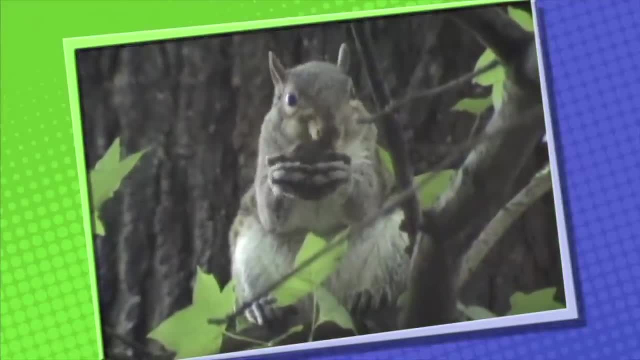 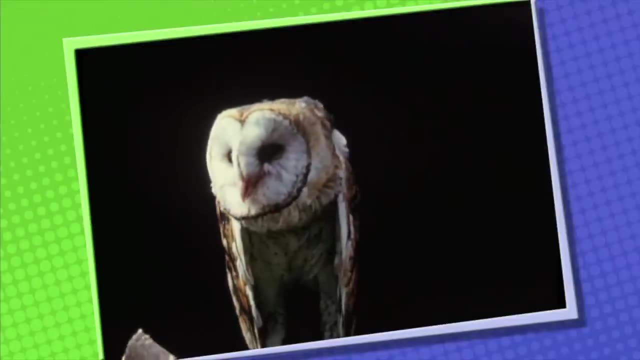 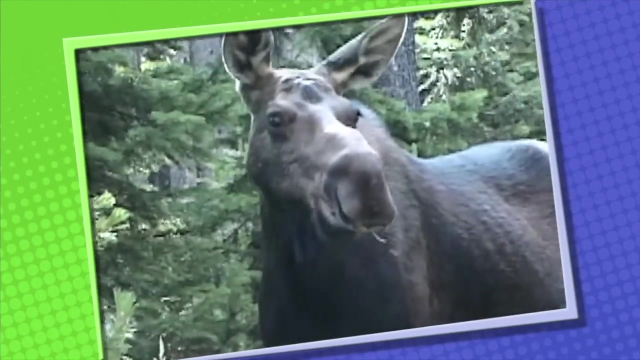 In coniferous forests you will find small animals like mice, squirrels and beavers. The branches of the trees offer shelter to a wide variety of birds, including owls. On the ground, you'll find large animals like moose, the largest member of the deer family. 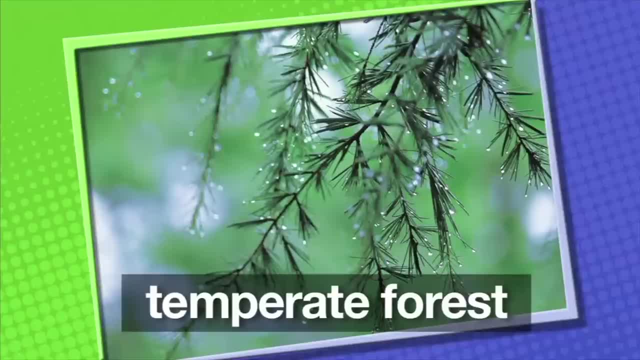 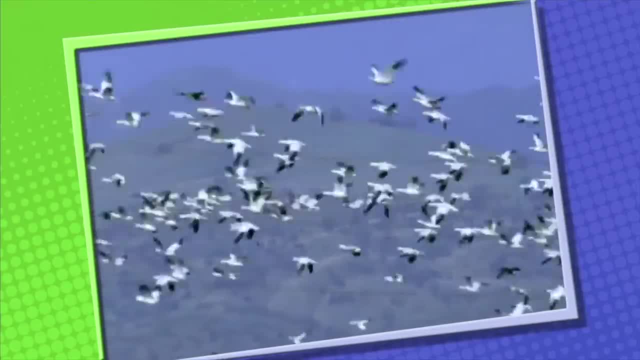 Temperate forests are found on the North American continent, South America, Europe, Africa and the United States. Skulls and birds who live in the temperate forests migrate to warmer places in the winter. Skulls and birds who live in the temperate forests migrate to warmer places in the winter. 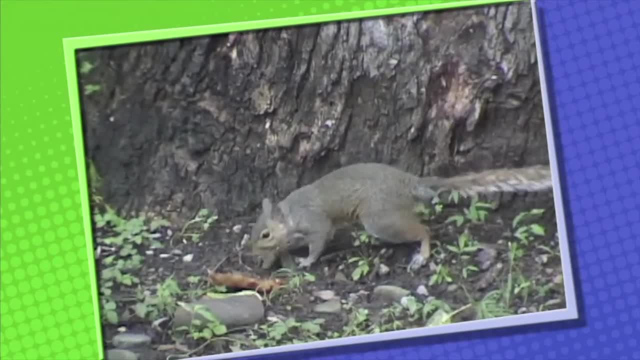 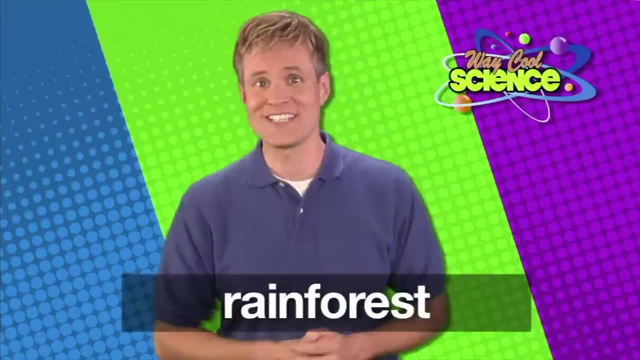 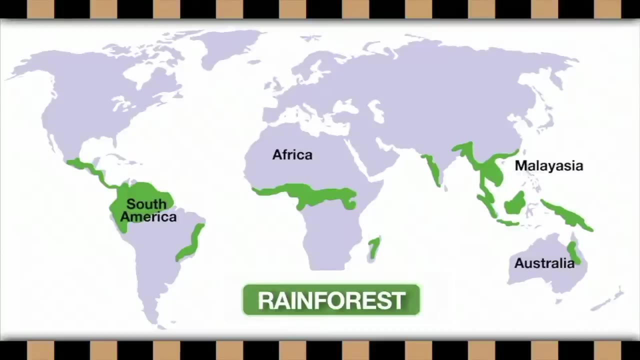 Squirrels adapt to the seasons too. They store nuts and acorns to eat in the winter. Bears sleep or hibernate through most of the winter. The third type of forest habitat is a rainforest. Rainforests are found in South America, Africa, Malaysia and Australia. 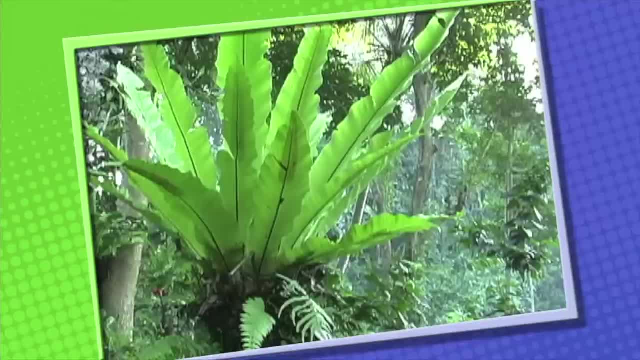 The plant in rainforests grow very quickly and they are adapted to the large amounts of rainfall during the winter. During the winter, high открывặc, comfortable trees, species infested rocks and green chocolate crops are found on the North American continent, South America, Europe, Africa and the United States. and the excessive heat that are characteristic of rainforests. In a rainforest, you'll find plants with very broad leaves and trees that grow tall above the shrubs and vines. Animals living in a rainforest have adapted to life among tall plants. 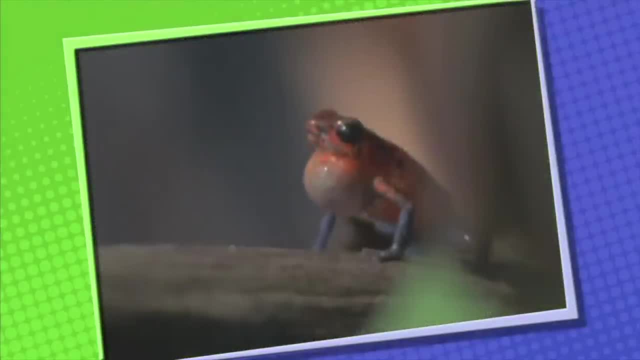 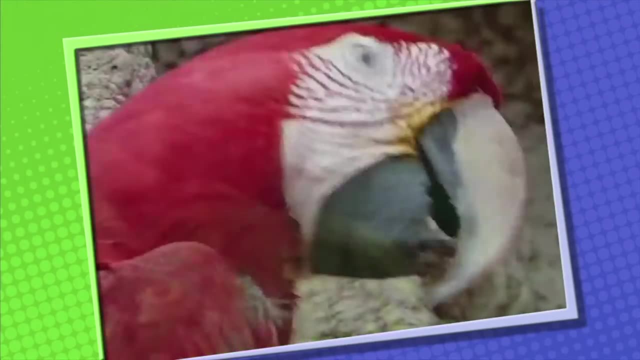 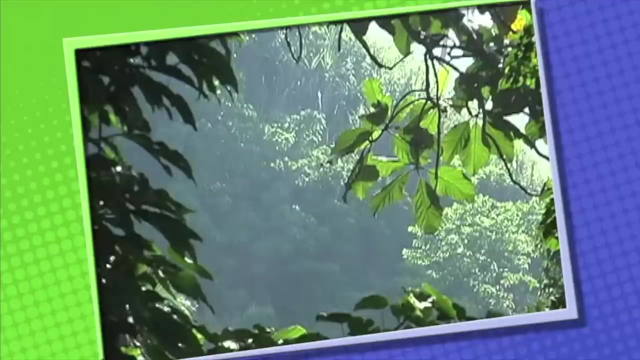 There are small animals like tree frogs. Large predators have body colors that help them to hide in the dense foliage, And the bright and colorful macaws blend in with the flowers of the rainforest. In addition, the rainforests have the largest insect population in the world. 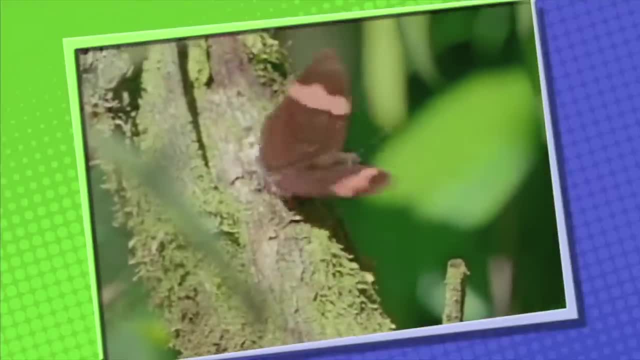 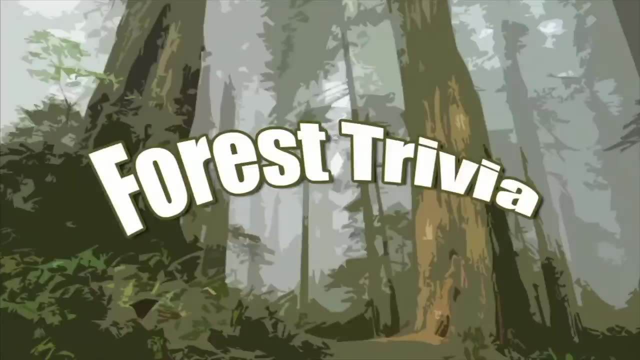 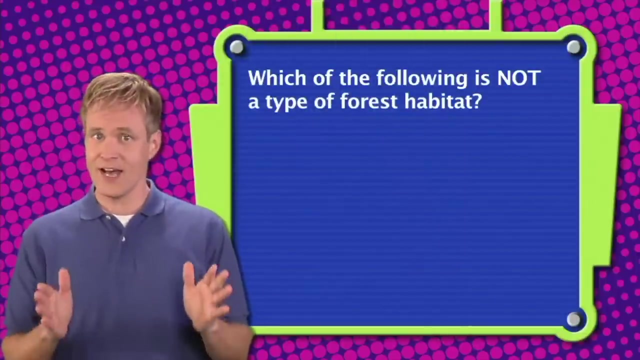 including one of the largest populations of butterflies. Okay, you're not out of the woods yet. It's time to play Forest Trivia. See if you can answer the following questions. First question: Which of the following is not a type of forest habitat? 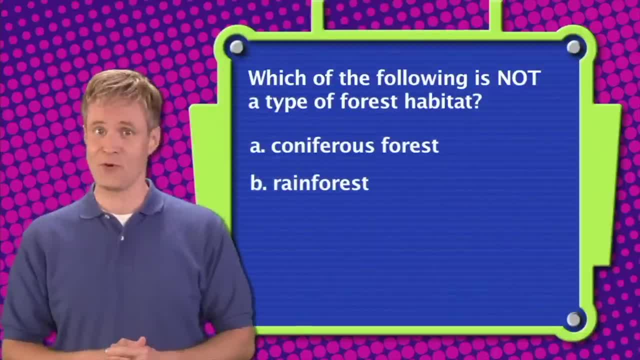 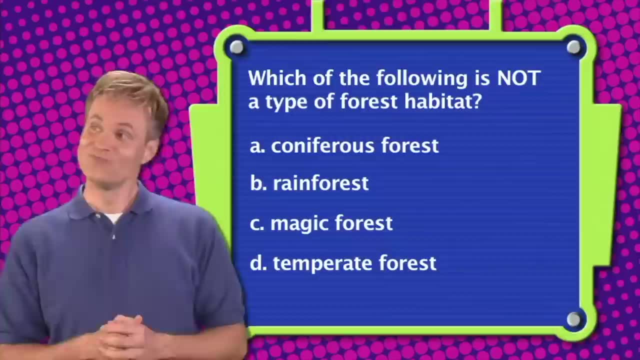 A- Coniferous forest, B- Rainforest, C- Magic forest Or D- Temperate forest. If you said coniferous rain or temperate forest, you're barking up the wrong tree. The correct answer is C. 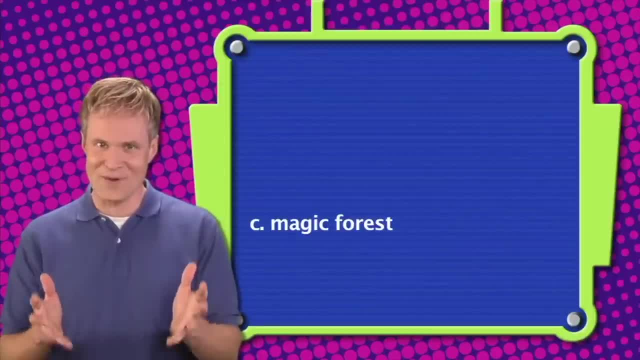 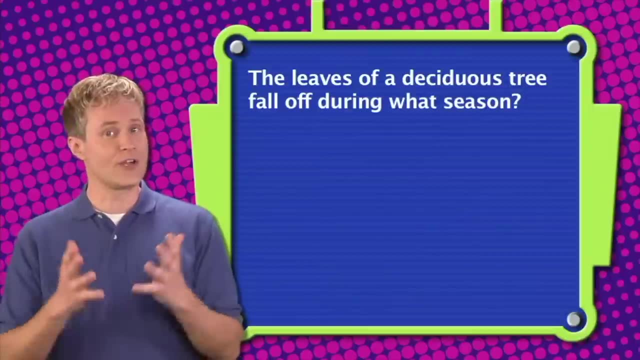 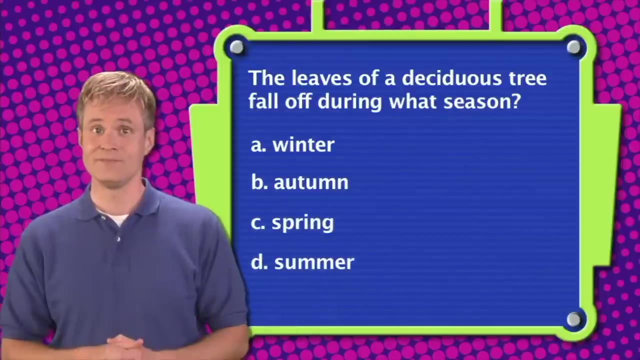 Magic forest is not a type of forest habitat. Here's the next question: The leaves of a deciduous tree fall off? during what season? A Winter, B Autumn, C Spring Or D Summer? The correct answer is B. 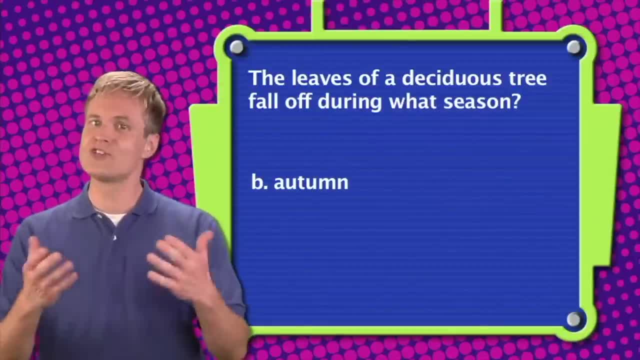 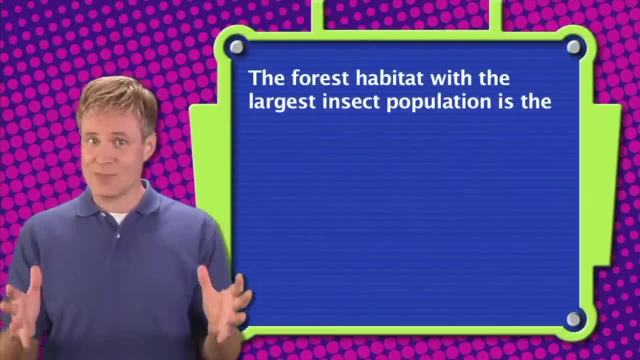 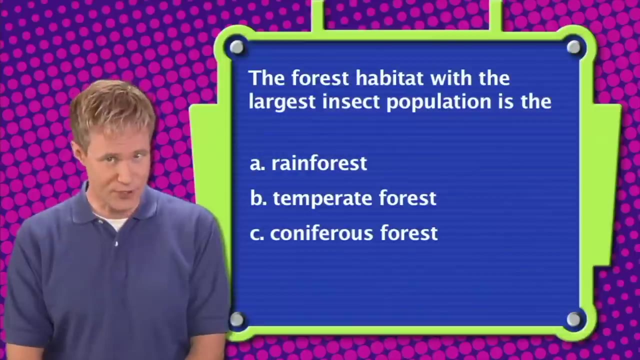 The leaves of a deciduous tree fall off during the autumn season. Here's our final question: The forest habitat with the largest insect population is the: A- Rainforest, B- Temperate forest, C- Coniferous forest Or D- All of the above. 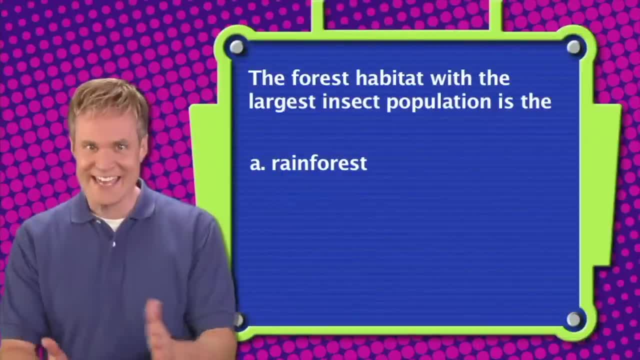 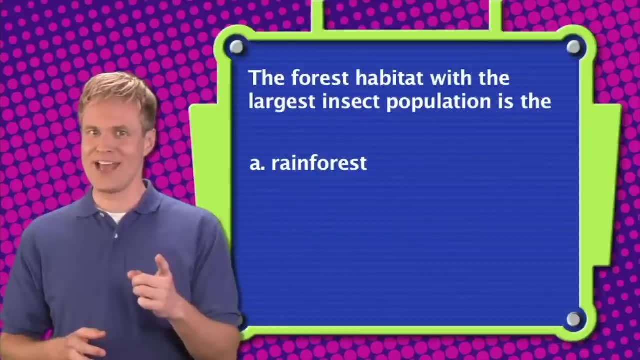 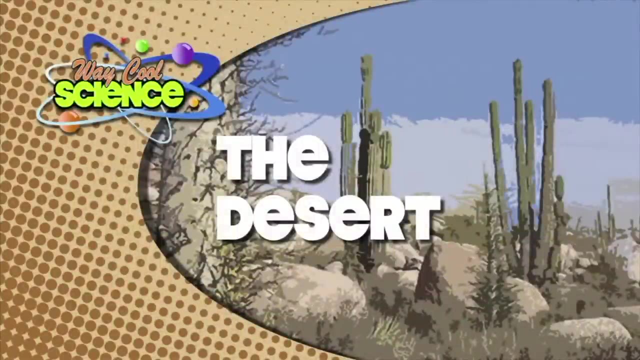 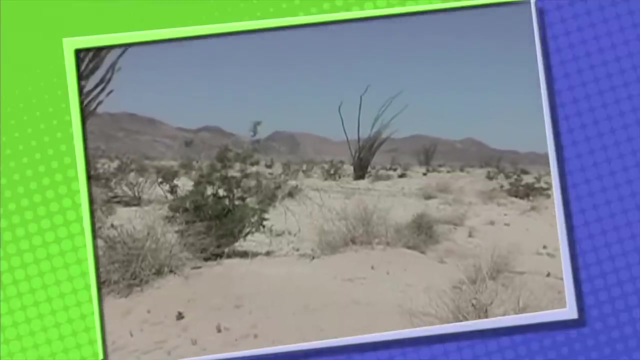 The correct answer is A. The forest habitat with the largest insect population is the rainforest. Thank you for playing Forest Trivia. The next habitat we're going to visit is the desert. The desert habitat can support very little life because there is very little precipitation. 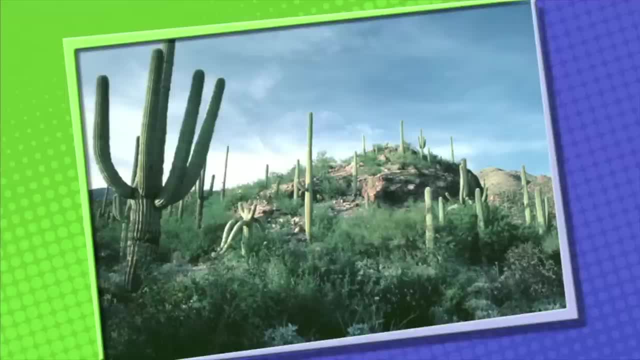 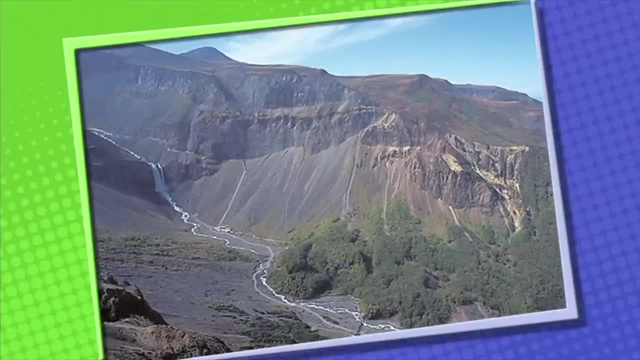 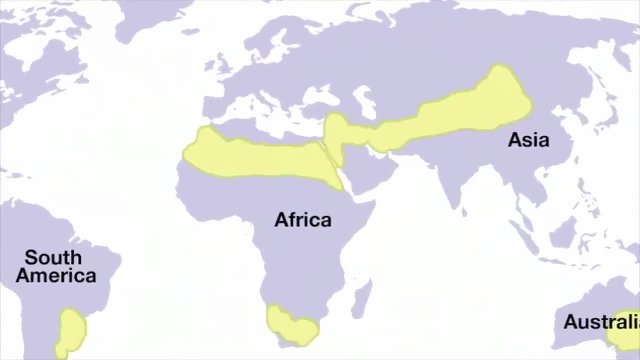 and therefore very little water. When you think of the desert, you might think of a very hot, dry place, But there are actually different types of deserts with different climates. One kind of desert is hot and dry. An example of a hot, dry desert is also the world's largest desert. 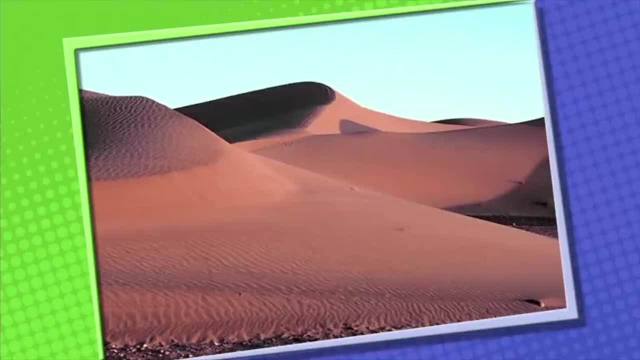 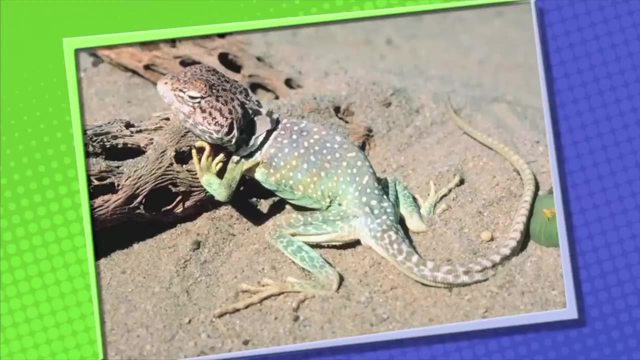 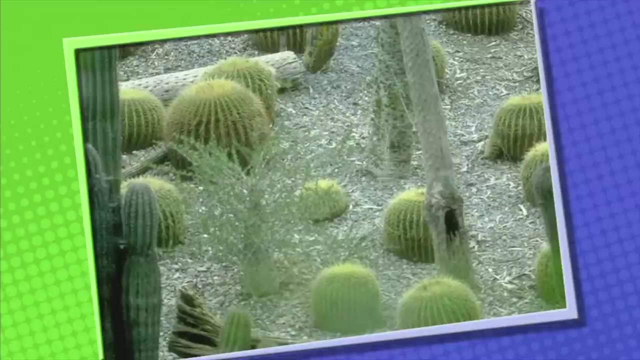 the Sahara in northern Africa. Another kind of desert is cold and dry, like the Gobi Desert in northern China. Each type of desert has its own plants and animals, all of which have adapted to low moisture conditions. In the hot desert you can find many different cactus species and some plants. A few animals are equipped to survive in a desert biome. A camel can live in a desert because it stores fat in its hump. When food is scarce, the fat stored in the hump allows the camel to survive for two weeks without eating. 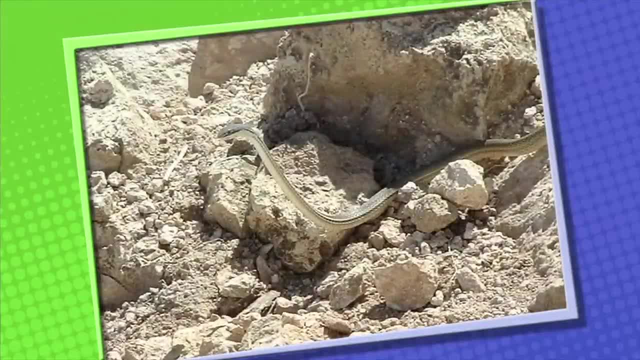 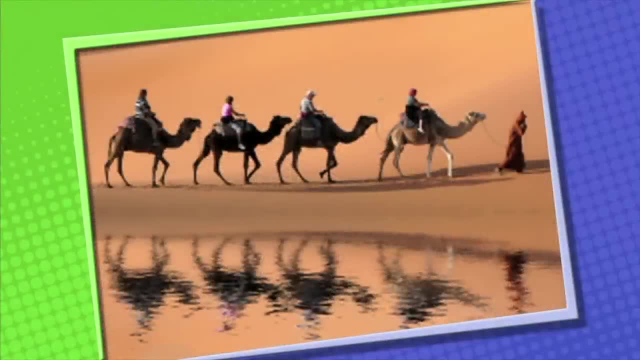 You'll also find a variety of snakes and strange animals like armadillos. Even though water is scarce, many people choose to live in the desert. One way people have found to live in the desert is to be a nomad or to be nomadic. 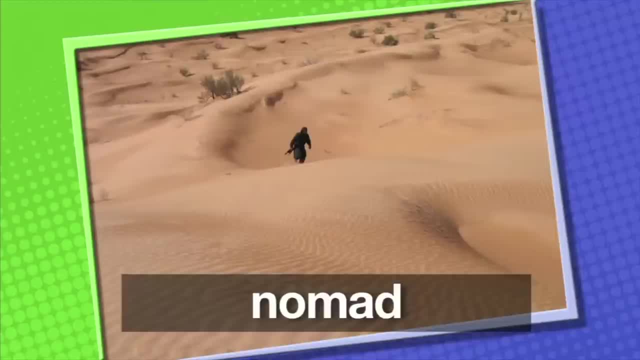 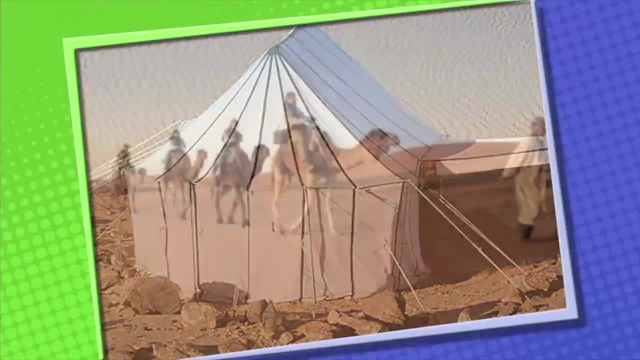 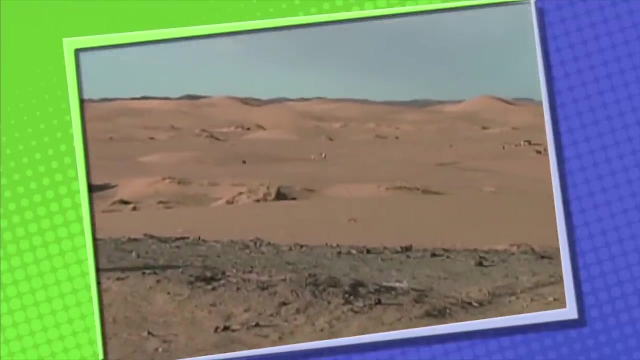 Being a nomad means that you have no permanent income and you have no money. You have no permanent home. You move from one oasis to another across the desert. Many nomads herd cattle, sheep or camels. By moving their flock, they prevent overgrazing of the sparse vegetation. 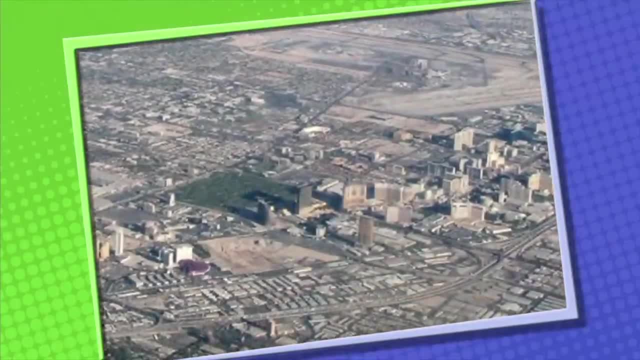 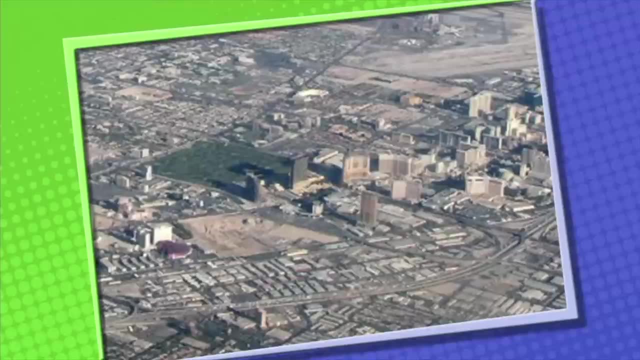 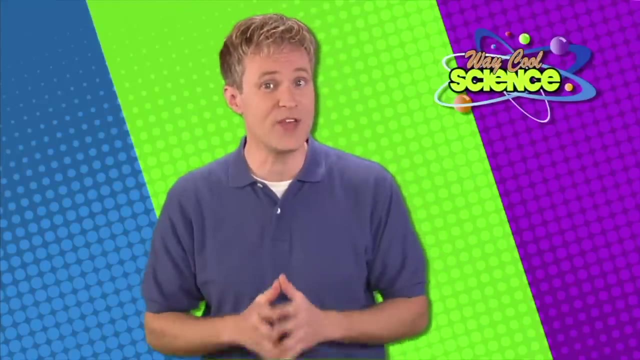 and exhausting water sources. Many US cities are built in the desert. Las Vegas and Phoenix would not be possible without water sources from hundreds of miles away. Did you know that deserts can be found on every continent? Deserts cover more than one-fifth of the world's land. 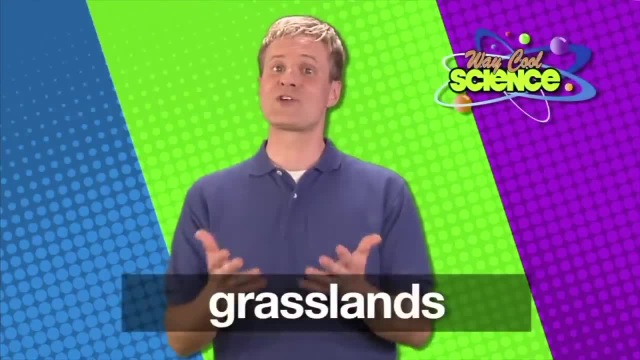 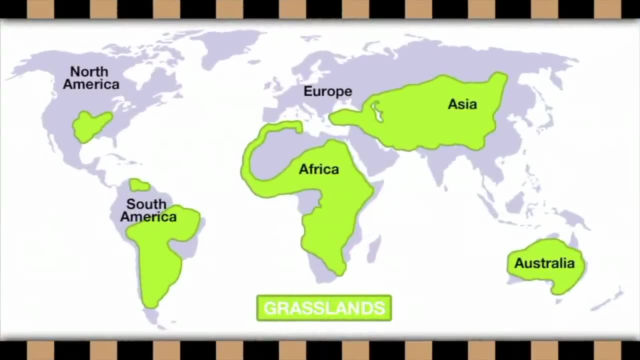 The next habitat we're going to talk about is called the grasslands. So fire up the Ryder mower and let's go. We find grasslands in North America and South America, Africa, Europe, Asia and Australia too. Grasslands are found on every continent. 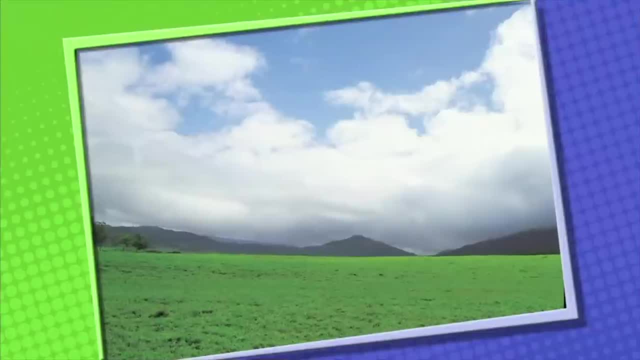 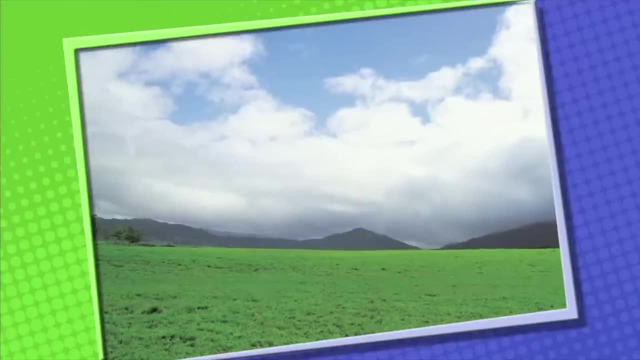 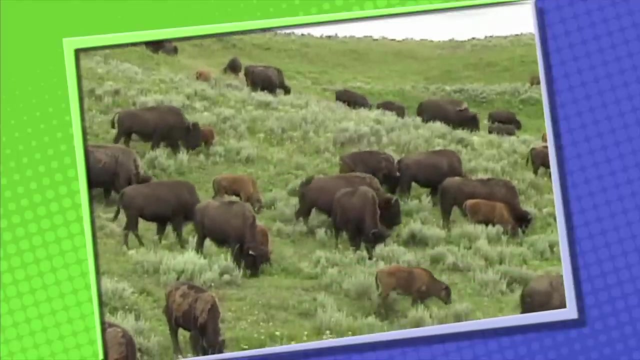 except Antarctica. Grasslands are typically large, wide-open spaces. Most plants found on the grasslands are grasses. There are very few trees found in the grasslands because there isn't enough rain. In the grasslands of North America you'll find large animals like buffalo grazing on the plains. 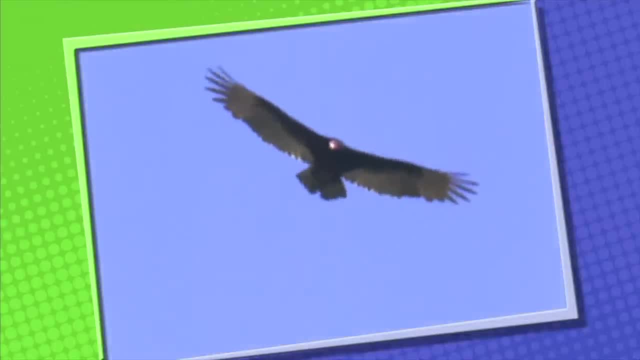 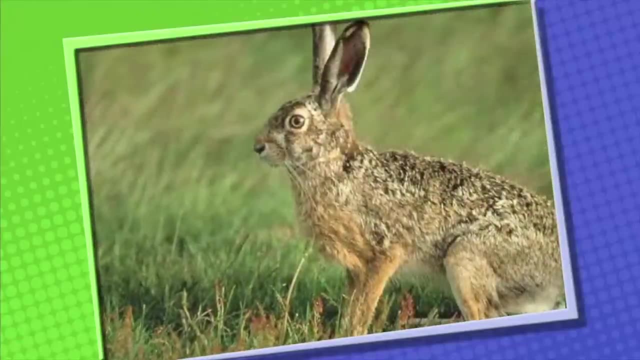 In the sky. you will find birds scanning the ground for small animals like rabbits. The grasslands afford animals very few places to hide from danger. Rabbits that live in the plains have adapted to life in the grasslands by having the ability to move very quickly. 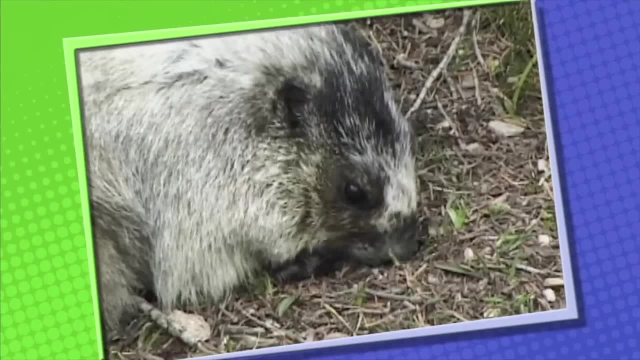 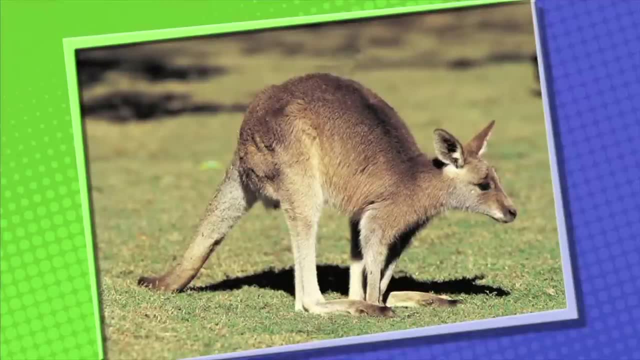 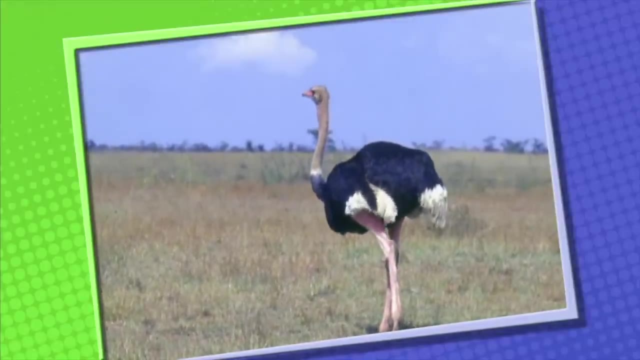 You'll also find a strange animal called a marmot, who digs furrows for protection from predators. On the grasslands of Australia, you'll find wallabies, a relative of the kangaroo, While in Southwest Asia you'll find a fast-running but flightless bird. 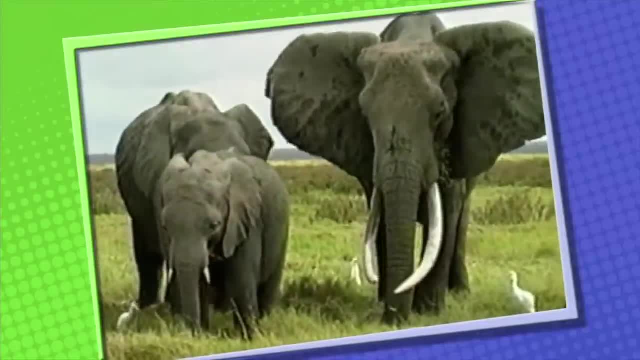 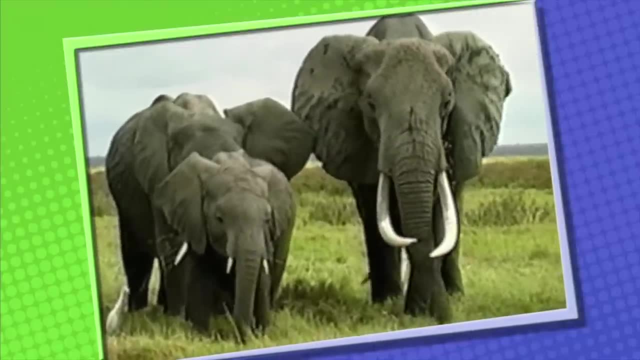 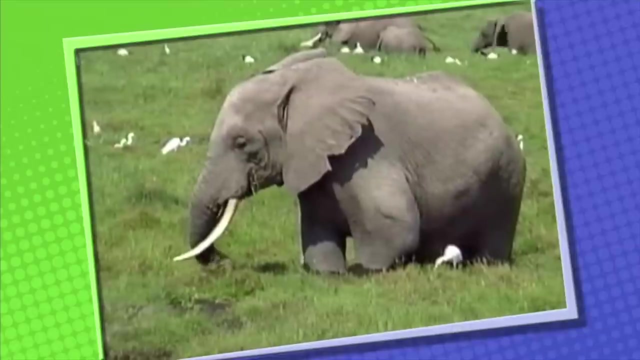 the ostrich In Africa, there are large grazing animals such as elephants. Elephants have adapted to the grassland habitat. The elephant's long trunk is very effective for carrying large amounts of water that can be transferred to other places during times of drought. 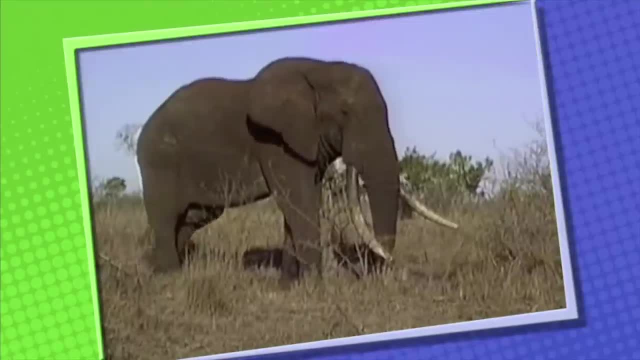 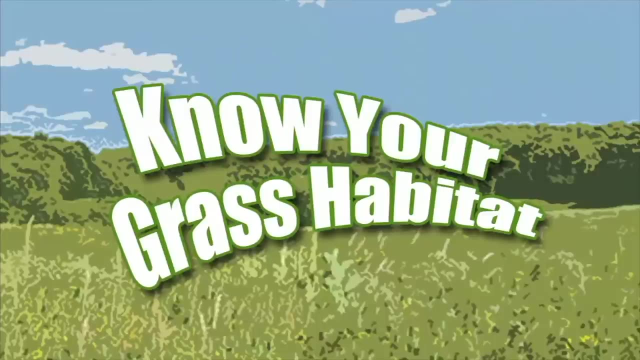 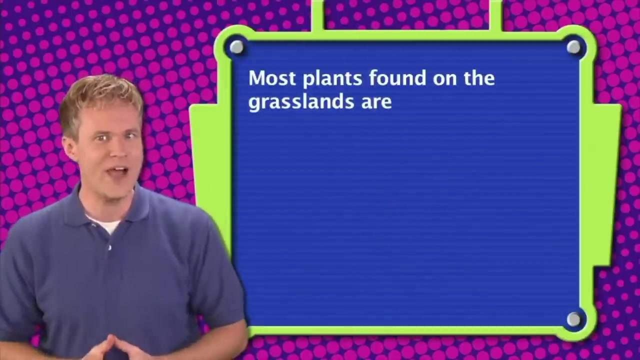 Elephants have sharp tusks to protect themselves from predators such as lions. Okay, it's time to play that non-allergenic, green and sassy, soft and grassy game. Know Your Grasshouse? Here's your first question. The correct answer is B. 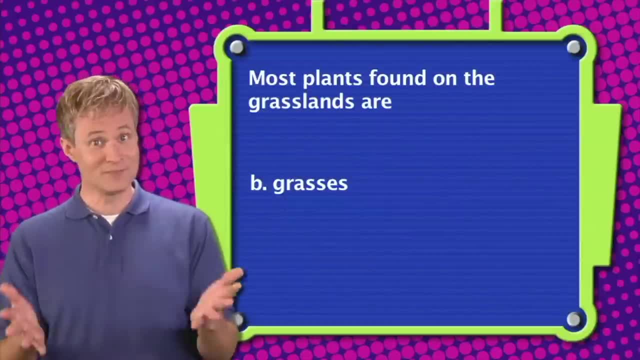 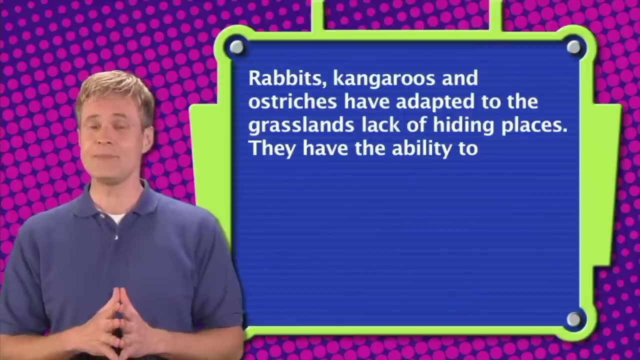 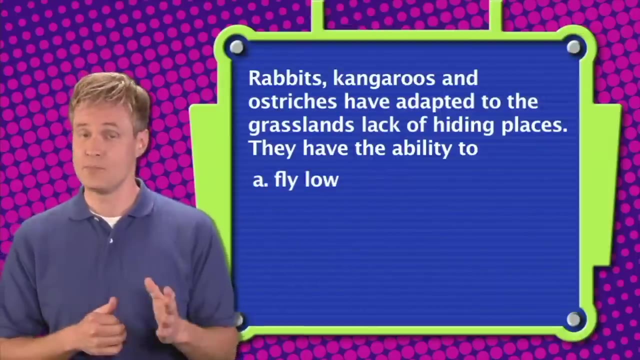 Most plants found on the grasslands are grasses. Here's your next question. Rabbits, kangaroos and ostriches have adopted the lack of hiding places around them. They have the ability to: A- Fly low. B- Move quickly. C- Eat grass. 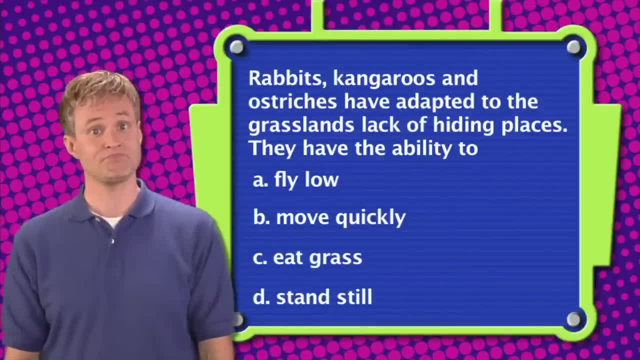 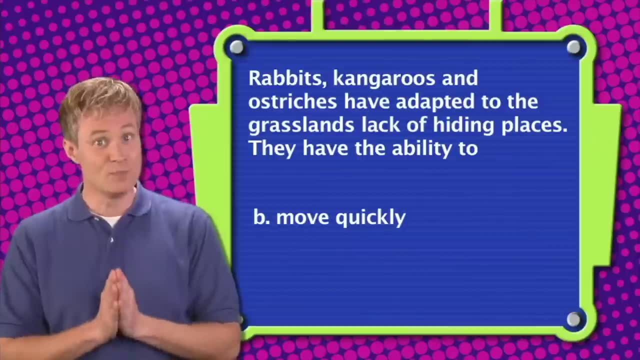 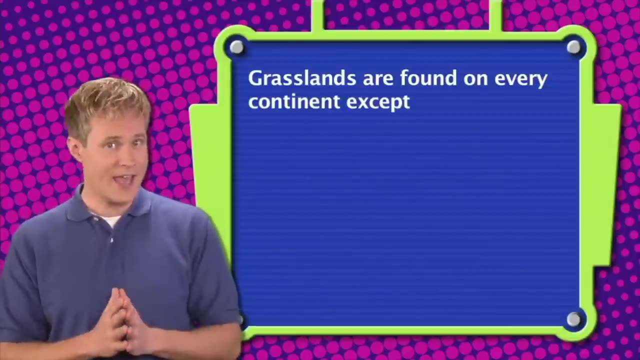 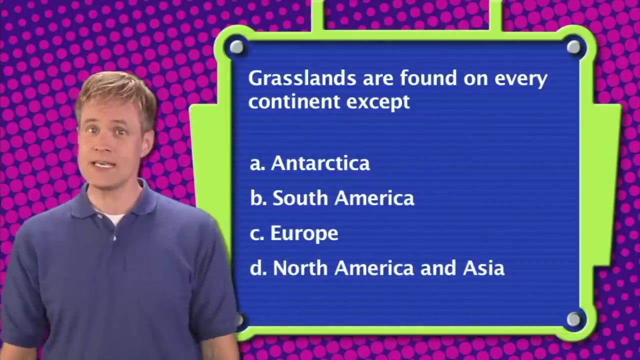 or D Stand still. The correct answer is B. They have the ability to move quickly. Here's your final question. Grasslands are found on every continent except A Antarctica, B South America, C Europe or D North America and Asia. 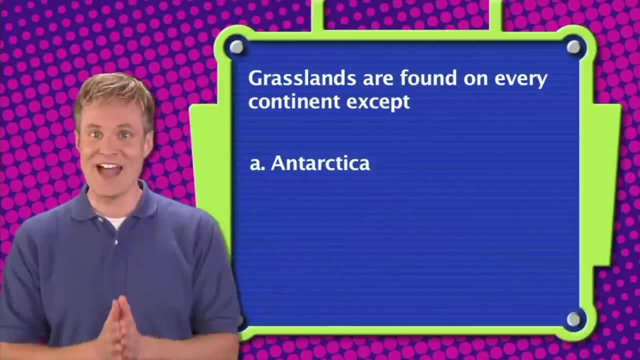 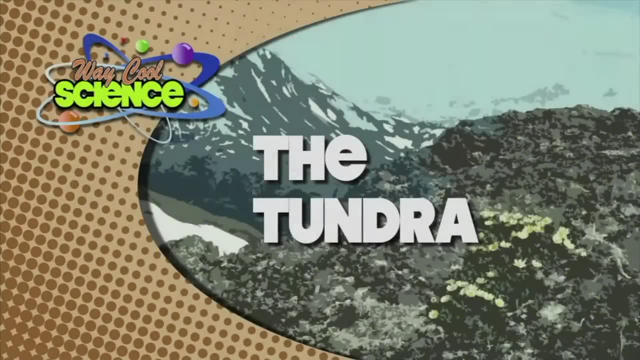 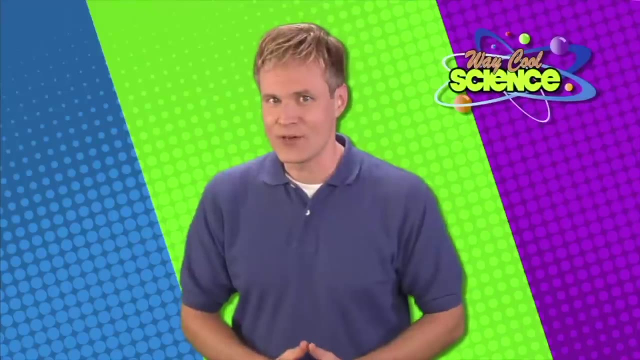 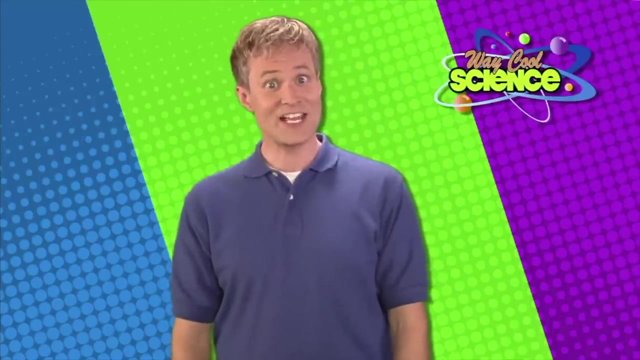 The correct answer is A. Grasslands are found on every continent except Antarctica. The next habitat we're going to visit is the tundra. It's a place that is cold, windy and dry. Sounds like fun. The tundra is found in North America, Greenland. 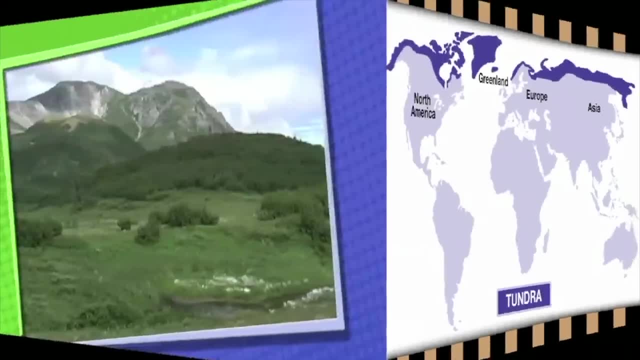 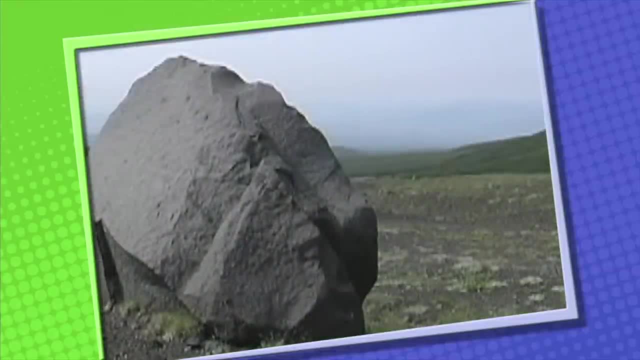 and parts of Northern Europe and Northern Asia. The word tundra comes from a Finnish word which means barren land. It was considered barren because there were no trees on the tundra, But there are some plants that have adapted to the cold and bleak habitat. 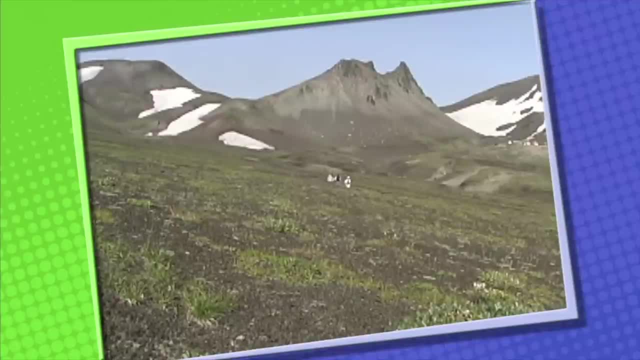 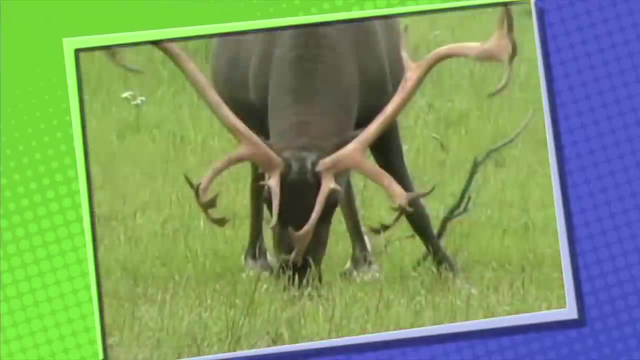 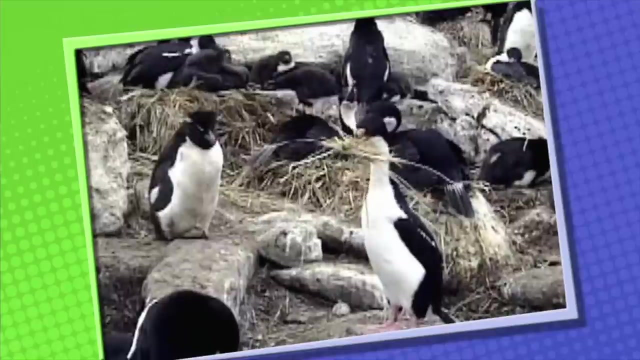 Those plants are mosses, grasses and small shrubs. The tundra habitat offers very little shelter from the weather. However, some animals do live on the tundra. They include caribou seals, brown bears and a variety of unusual birds. 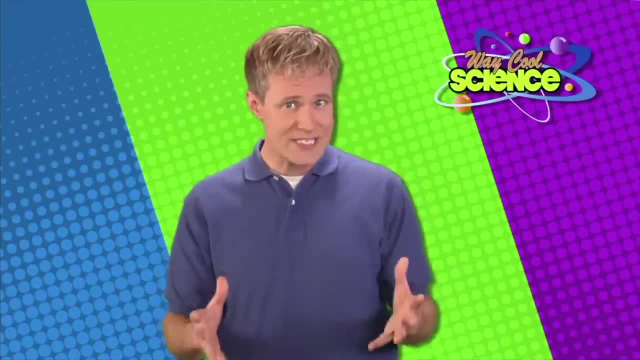 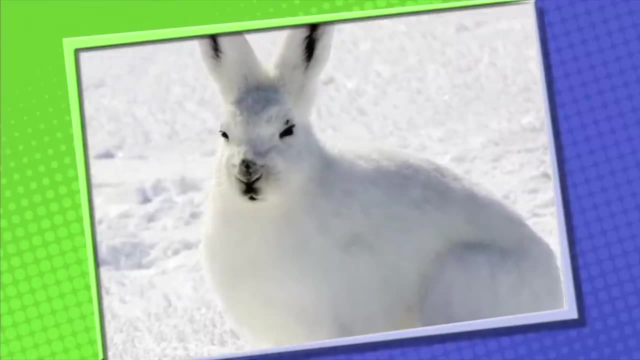 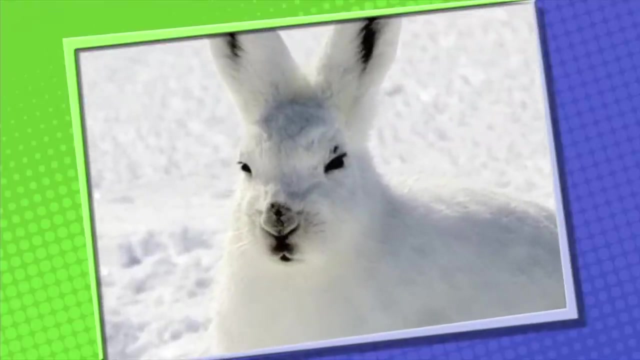 Some animals who live on the tundra have adapted to the seasonal changes of their habitat by changing the way they look. For example, the arctic hare protects itself by changing to a lighter colored fur in the winter. The light colored fur helps it to blend in with the ice and snow to protect it from predators. 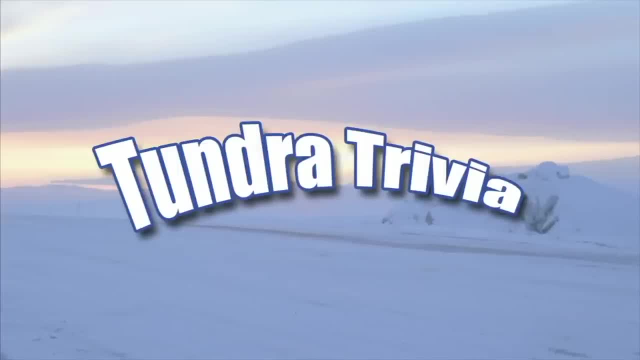 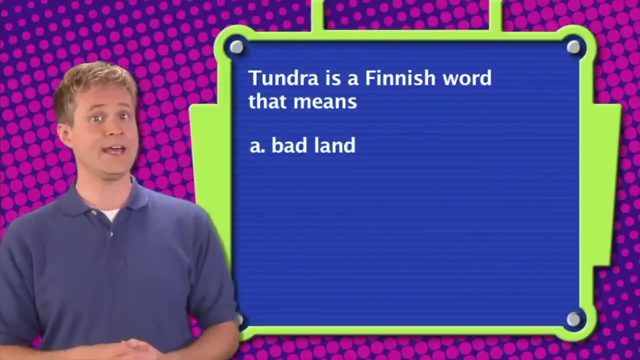 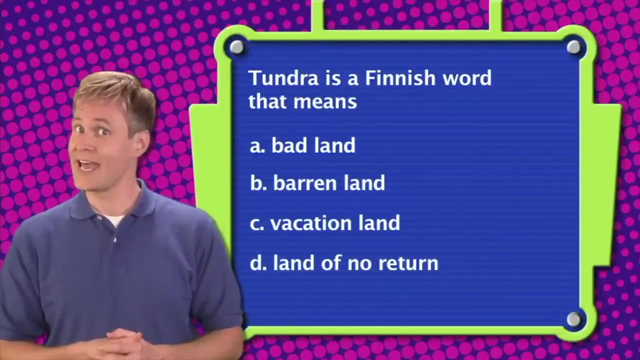 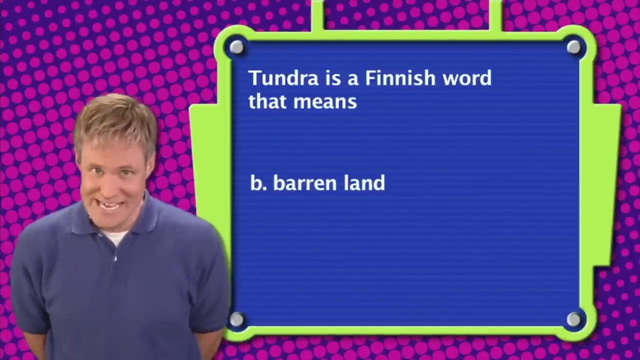 Okay, now it's time for tundra trivia. Here's the first question. Tundra is a Finnish word that means A- Bad land, B- Barren land, C- Vacation land or D- Land of no return. The correct answer is B. Tundra is a Finnish word that means: 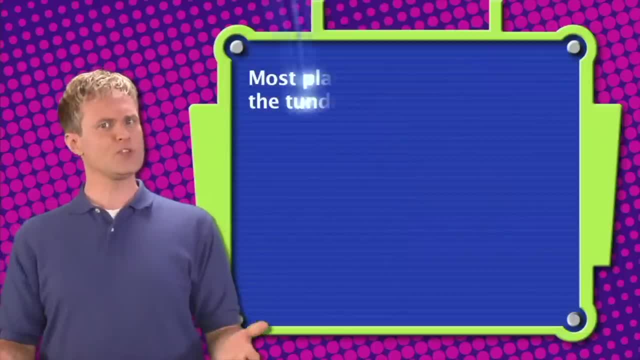 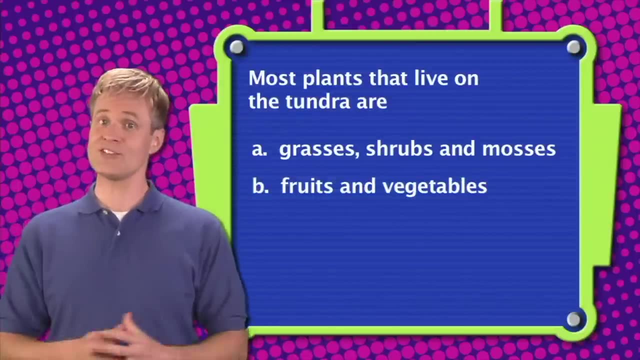 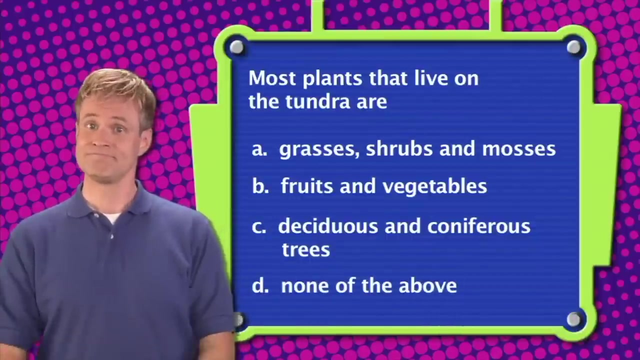 Barren land. Next question: Most plants that live on the tundra are: A- Grasses, shrubs and mosses, B- Fruits and vegetables, C- Deciduous and coniferous trees or D- None of the above. The correct answer is